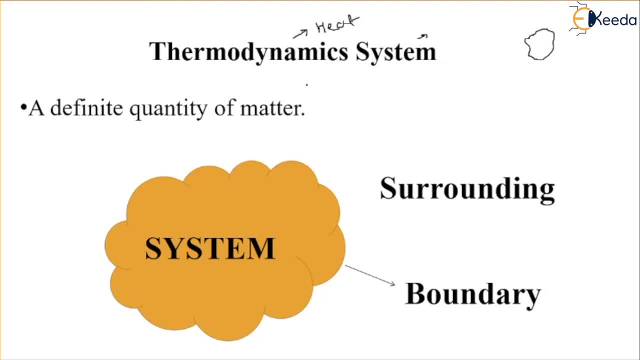 that is called the system, And thermodynamic system is what Any system which is under the application of heat. So thermodynamic system we can define as a quantity of matter in space which is subjected to any kind of heat or which is subjected to temperature and temperature. 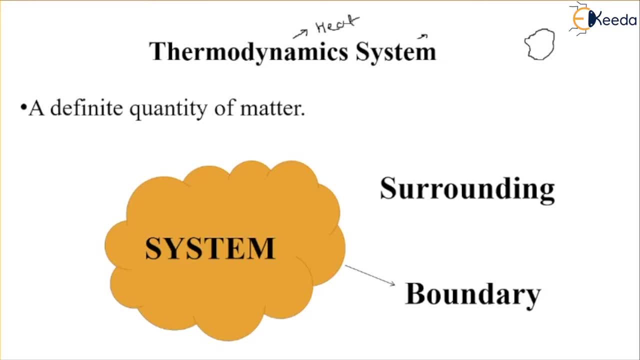 difference. So this is the basic definition of system. So in simple word we can say system is a definite quantity of matter. If we say simple definition of system and thermodynamic system, which is related to temperature, temperature difference, heat, heat transfer and transfer of energy into work, These terms are involved. So here this: 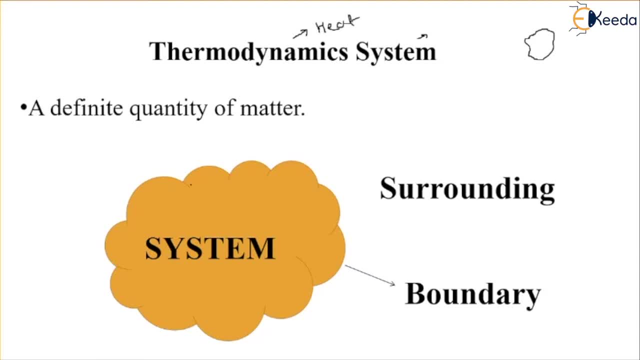 particular diagram you can see. this diagram is representing a system. It means it is a kind of body. So this is a closed object. and external to this closed object, whatever you can see, that is the ceramic suppose, if you are standing in a ground, so, and there is nothing in the ground, so for that. 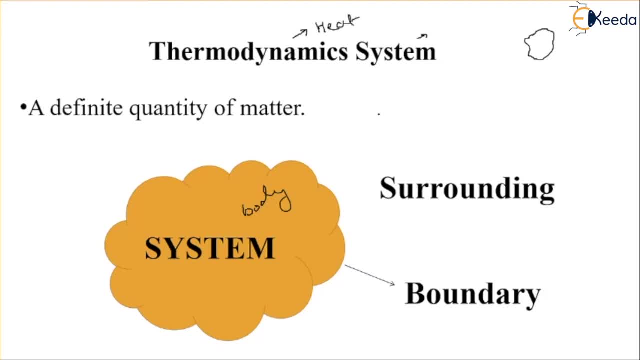 particular condition. you are the system and around you everything is surrounding. suppose you are in a swimming pool, or if you are in a river, and if you are swimming in a river, so in your surrounding, what other thing which we, we can see, that is the water only. so for that particular condition you 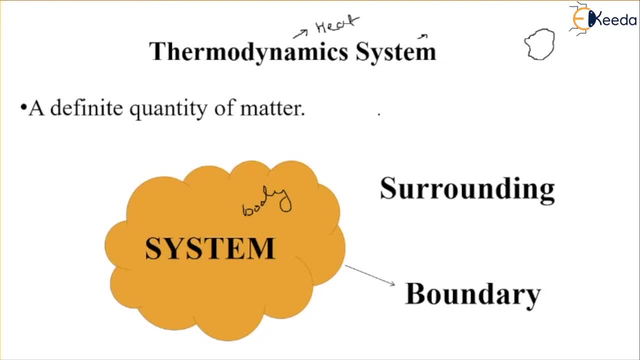 are the system and the whole water is the surrounding. so this is our system, which is made up of definite quantity of matter. this is representing the system, and everything else around the system is called surrounding, and the thing which is differentiating this system and surrounding it is called the. 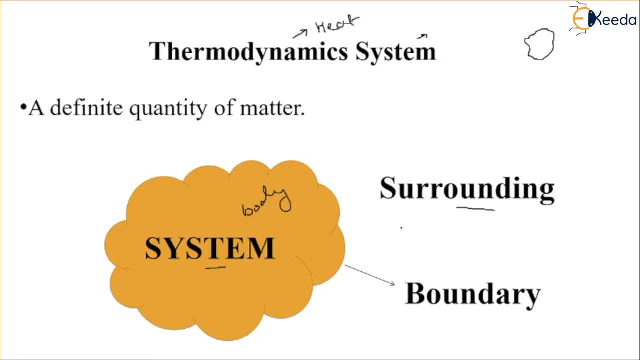 boundary. so in simple word we can say: system and surrounding, both are separated by the boundary and this boundary can be fixed or it can be moving type. the boundary will not always fix. it can be fixed or it can be a moving type of boundary. and all these things- system surrounding and the boundary which is separating system and surrounding. 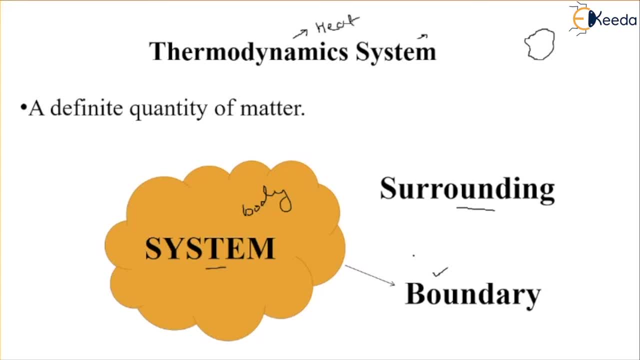 boundary. if we combine all these things, it is making the universe. So this is the basic definition of system surrounding and boundary. Now here, when we apply temperature application or heat application, so the system will become thermodynamic system. Now let's discuss the basic types of thermodynamic. 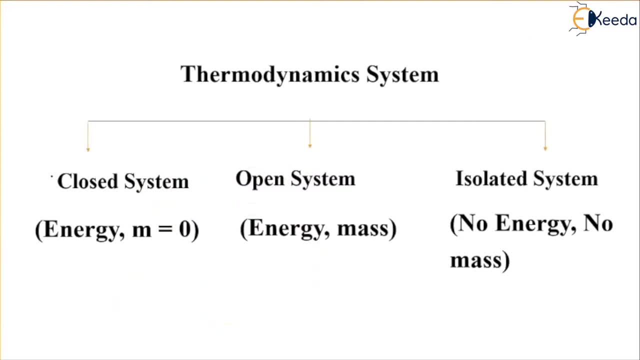 system. So there are three types of thermodynamic system we consider: One is the closed system, other is the open system and third is the isolated system. So, one by one, I will discuss these things here. So, as you can see, it is written here in front of closed system. 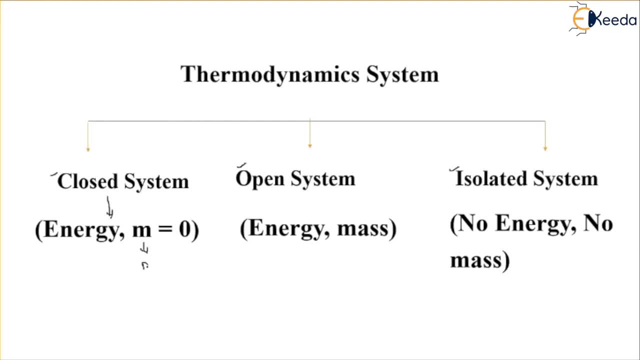 m equals to 0. So this m is representing the mass. So m is 0 means there is no mass. So this is not true. Mass will not be 0, but the transfer of mass will be 0 inside the system. But energy transfer is possible. Now in open system, mass transfer is possible as well as. 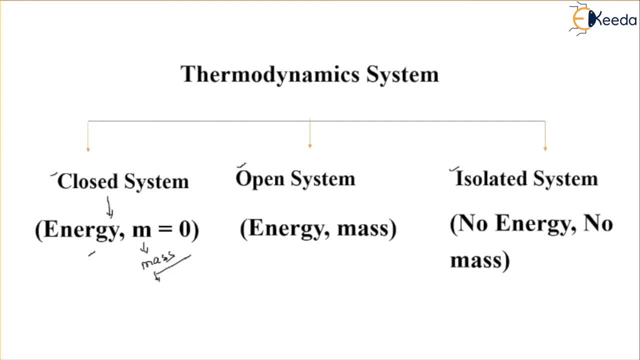 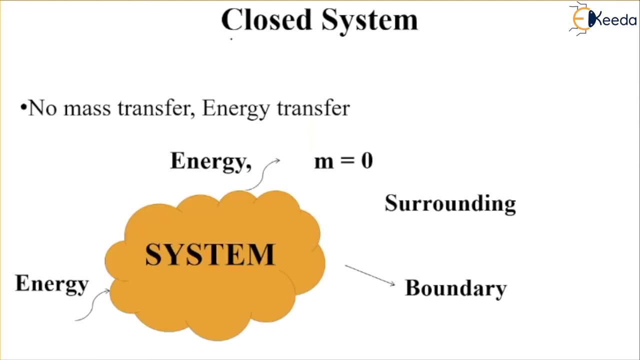 energy transfer is possible. Now in third type of system, isolated system, neither energy transfer nor mass transfer is possible. So these three types of system we have to learn. Now let's discuss one by one about these kind of systems. So first I will discuss about 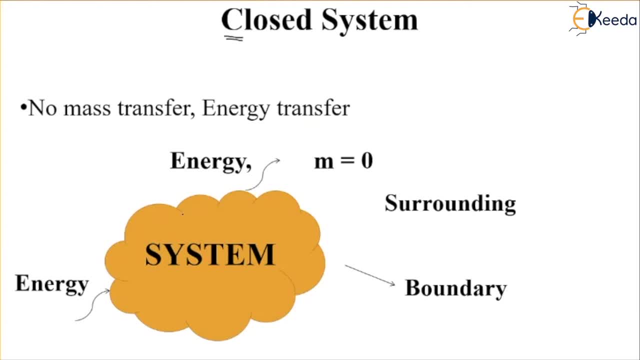 the closed system In closed system. you can see this diagram. So this particular diagram is representing a system which is made up of fixed quantity of matter. It can be anything. The system can be anything. Now, here you can see if we want to transfer the mass from this side to. 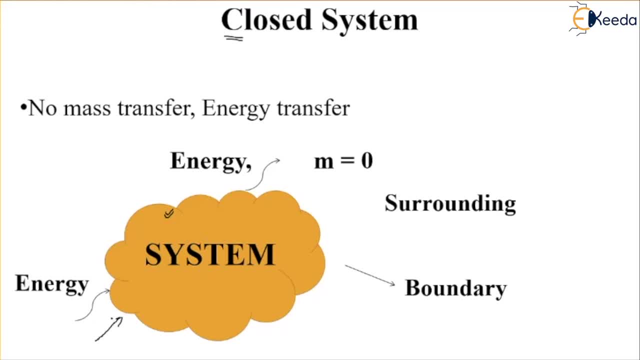 or if you want to enter some mass inside the system and the mass is not entering and this mass is also not leaving the system. So this particular type of system is called closed system. There is no transfer of mass from the system to the surrounding as well as 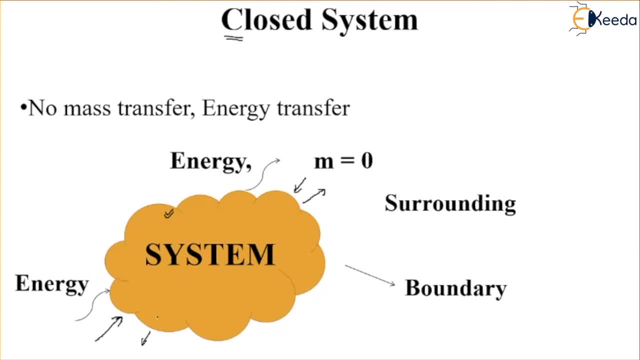 from surrounding to system. This particular system is called closed system right, And so here the mass transfer is not possible. But if we want to transfer the energy, so energy transfer is possible from system to surrounding and from surrounding to system. So 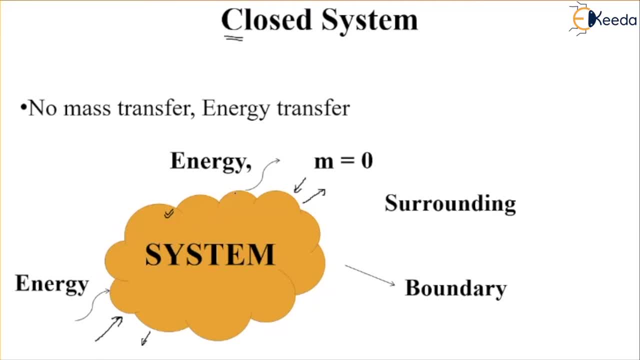 this is also considered as closed system. Across the boundary, this transfer will happen. So what is closed system? Mass transfer is not possible from surrounding to system or from system to surrounding, But energy transfer is possible from system to surrounding and surrounding. So this is also considered as closed system. So this is also considered as. 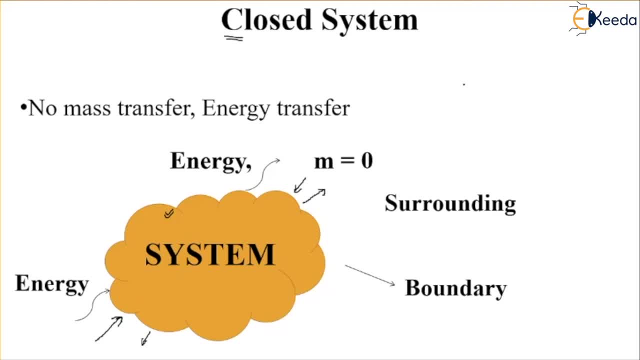 surrounding to system, So this is called closed system. Suppose: if you have a closed container which is filled up of water, This container is filled of water. Now if you are providing heat or if you are applying some temperature over this object, So what will happen, since this is a closed? 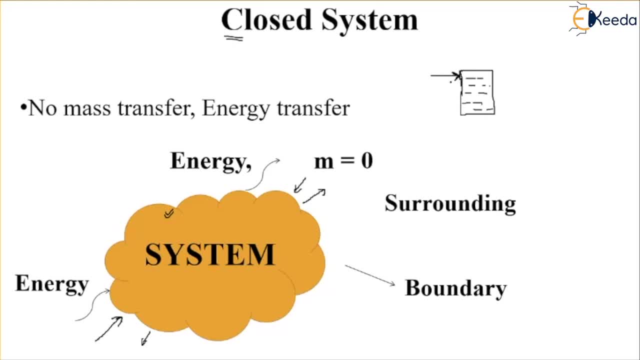 container. In that case heat will transfer into the system and it will heat this water and the temperature of water will increase. But since this particular object is completely closed, so this particular water which is converting into steam will not go away from this particular closed object, It will not come out from the object. 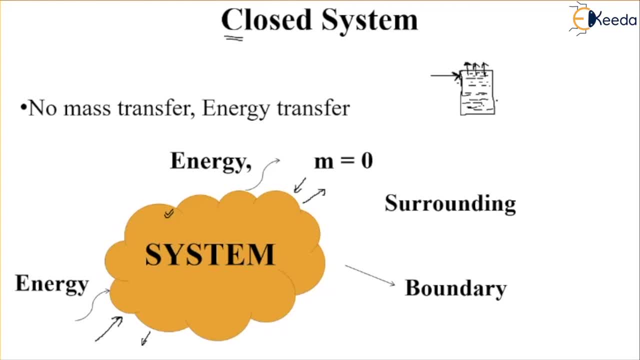 But heat will transfer from here to surrounding, Surrounding, to system. the heat is transferring, or the heat we consider as the form of energy. So energy is transferring and if we are removing this particular temperature application, So from system to surrounding, this heat will transfer. 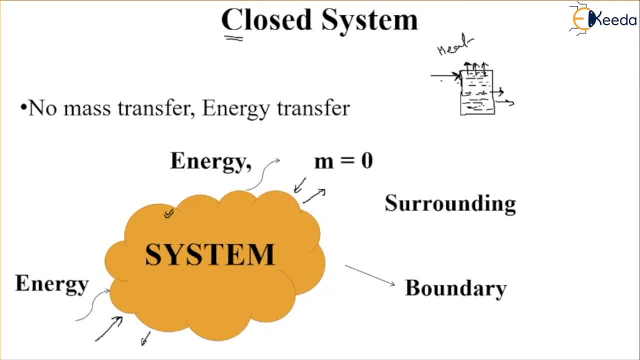 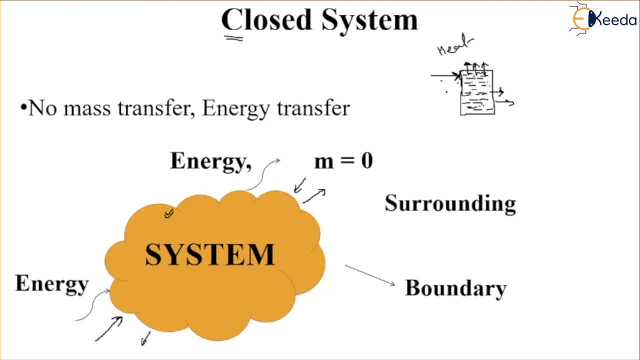 needed concentration of this object. So there are some more communication terms used here. So another point. so total charging, the system for not changing the volume here To remove the water or to remove the steam, so the volume of the water will not change. So here there is no mass transfer happening, or we are not. 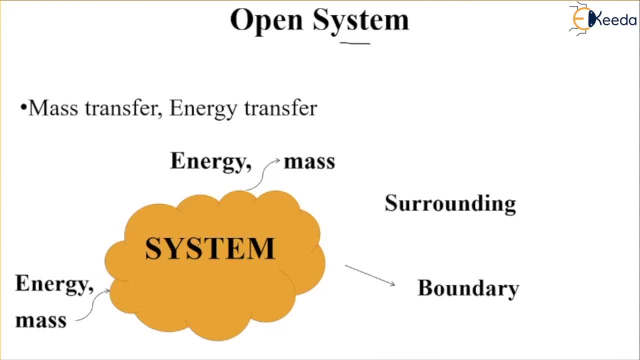 adding any kind of other matter or any kind of water inside this particular object. so there is no mass transfer is possible. but in terms of heat the energy transfer is possible. So this is called a closed system. suppose this is our system and if we want to transfer the mass inside the system from the 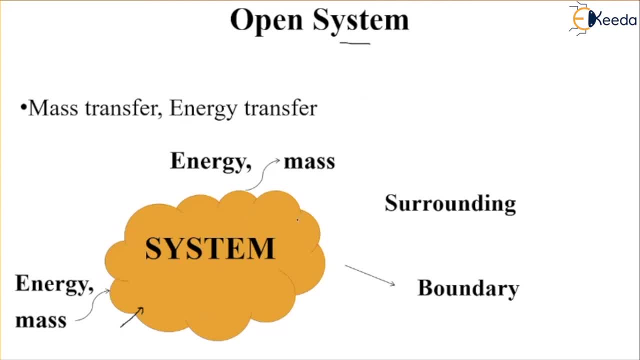 surrounding, or if we want to transfer the mass from system to surrounding. So it is possible. So mass transfer can be possible from system, and mass can be enter into the system from the surrounding. So this particular kind of system is called open system. Now let's come to the energy. 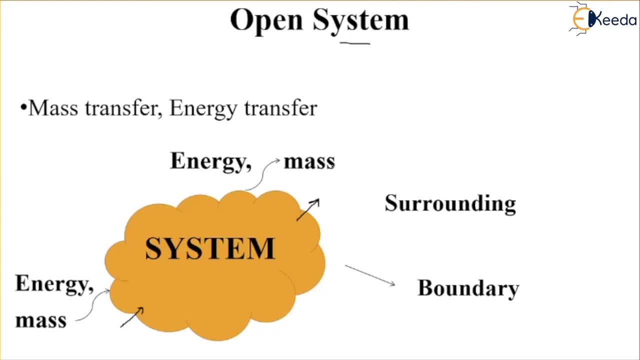 So energy transfer is also possible from system to surrounding or from surrounding to system. So this particular system is called open system. Here mass transfer is also possible and the energy transfer is also possible. Suppose we have any object or any container which is connected with one pipe and we are filling water inside this container. 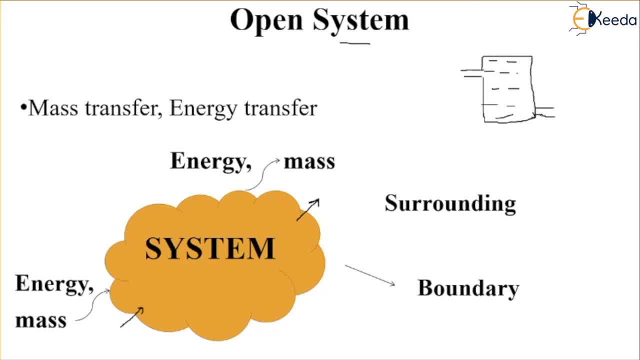 and there is some outlet. also, we are providing and the water is entering from here and the water is leaving this container from here. So this is the entry point and this is the outlet point and simultaneously we are providing heat to the container. So here the mass of the 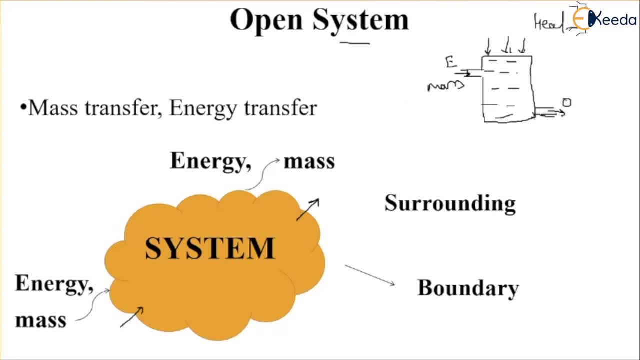 water is entering inside the container from here and leaving from the container to the surrounding, So the mass transfer is possible here as well, as heat is also transferring in the form of energy inside the container as well, as when we remove this heat application, So it will leave the 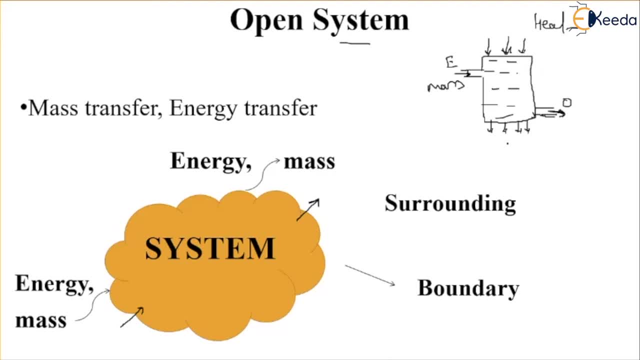 container. also it will leave the heat into the surrounding. So everything is possible. mass transfer is possible from system to surrounding or surrounding to system, as well as heat transfer or energy transfer also possible. So this is called open system. If we see any example of open system so we can say: 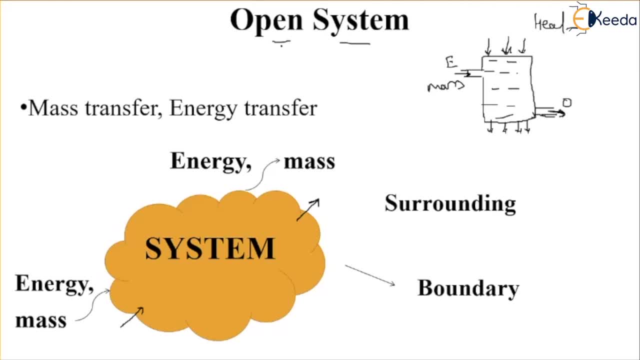 air compressor. So in air compressor air enter at the low pressure and it will also out at high pressure, And in air compressor energy transfer is also possible across the system boundary. So air compressor is one of the example of open system. Steam turbine can be considered as the 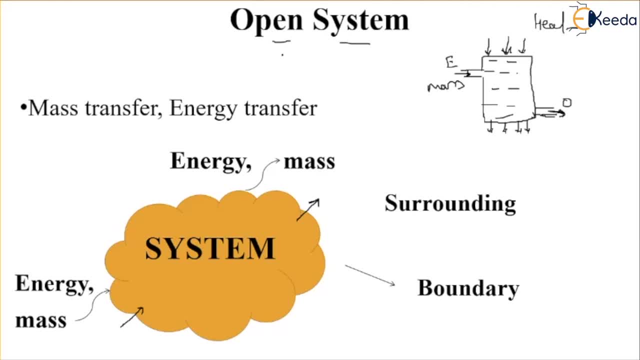 example of open system. There the heat transfer is possible inside the system and from the system to surrounding as well. as the water is circulating, It is converting in the heat and it is converting into the steam, and the steam is again converting into water and coming to the boiler. So circulation 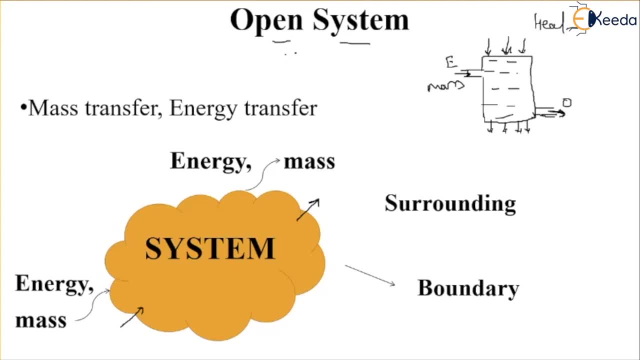 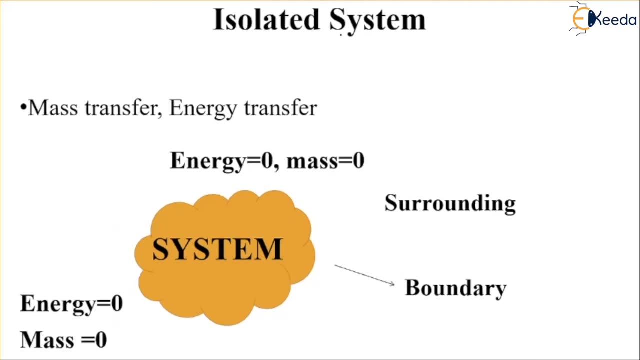 is continue from water to steam and from steam to water because of different processes, as well as heat, application is also there, So turbines are also considered as the example of open system. So this is about open system. Now, if we see isolated system, so this is the third type and 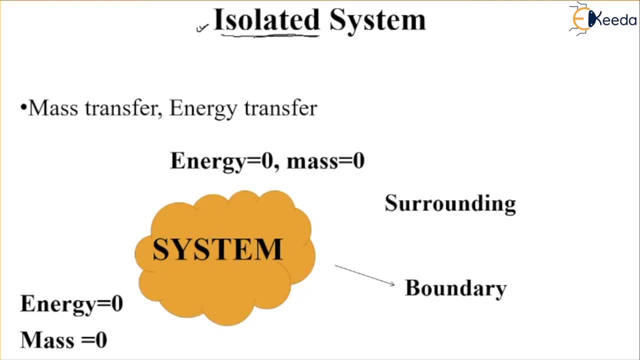 you can see the word isolated. Isolated means there is no transfer. So if we see any kind of system and if we are providing insulation to the system, suppose we are insulating this particular system. So in that case if we provide heat, so heat will not transfer. So if we provide heat, 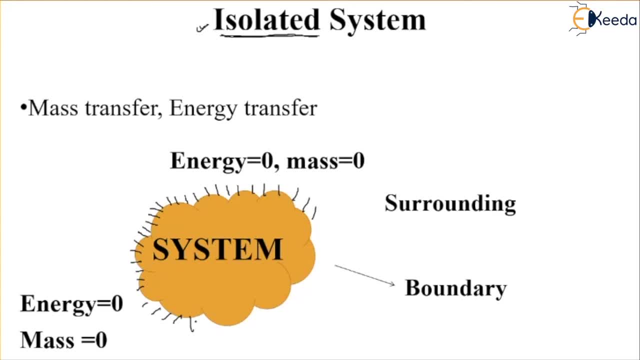 so heat will not transfer from surrounding to system because of the insulation, and if we are not able to transfer the mass from system to surrounding or from surrounding to system. So here neither energy transfer is possible nor mass transfer is possible. So mass transfer is zero. 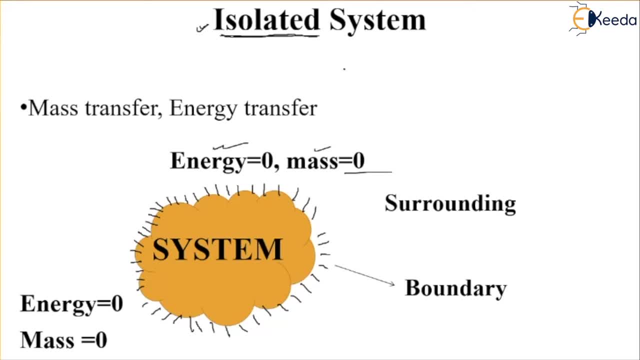 and energy transfer is also zero. That particular system is called isolated system Here, as I told you about the container which is filled of water. So this is the system. So if we have a water or any kind of liquid and if we are insulating the surface of this container, this surface of the 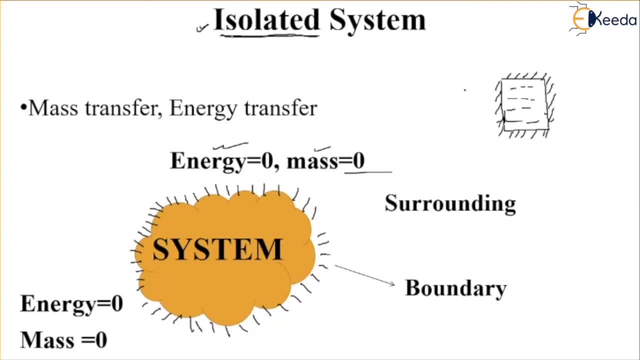 container is heat insulated. In that case heat will not transfer. Heat will not transfer from surrounding to system and if we are not applying heat, so it will not come out from system to surrounding as well. as this is completely closed system, So we cannot put any kind of mass in. 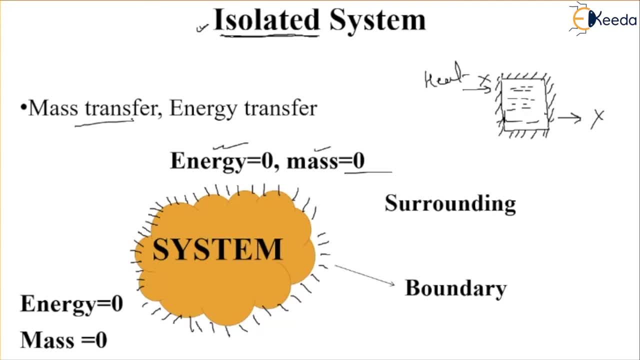 inside the system. So here neither mass transfer possible nor energy transfer possible. Here no mass transfer and no energy transfer is possible from system to surrounding or from surrounding to system. So this particular system is called isolated system. So here this particular system we can define as closed system with no energy, Closed system with 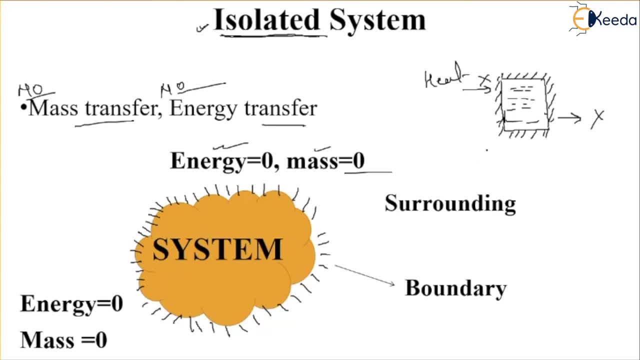 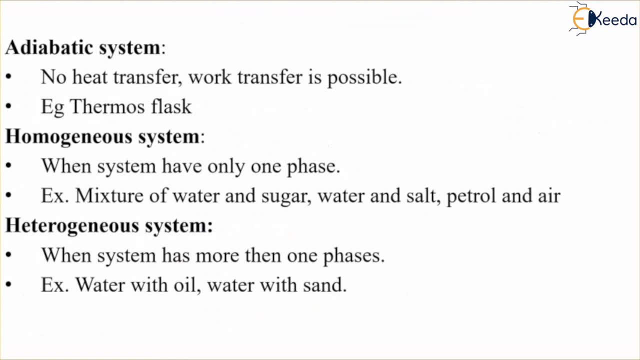 no energy. So these three types of systems we have to learn in thermodynamics. Now let's see some more types of thermodynamic system. So in this category the next thermodynamic system is adiabatic system. So adiabatic term we generally define with Q equals to zero, Q equals to zero. 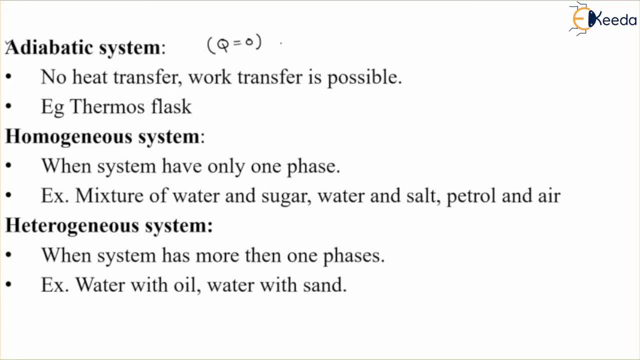 means there is no heat transfer from system to surrounding or from surrounding to system. So this system we usually define when there is no heat transfer from surrounding to system or system to surrounding. So that particular system is called adiabatic system. But here 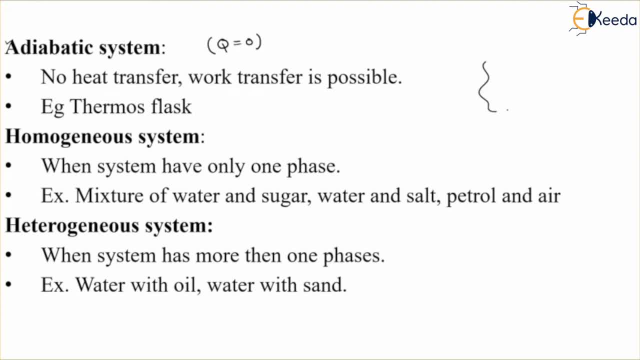 work transfer will be possible. So if we consider here a particular system, this is our system. So neither heat is entering into the system nor heat is coming out from the system. So no heat transfer is possible in this particular system. So usually we provide. 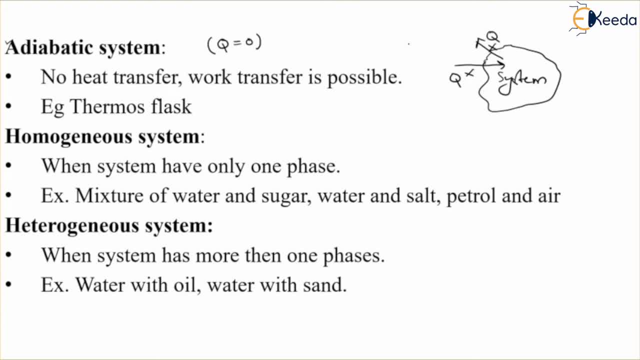 insulation in different types of systems, So that insulation is defined as the adiabatic system. But here work transfer is possible. So work can be transferred from system to surrounding or from surrounding to system. So this type of system is called adiabatic system. Example we can take as: 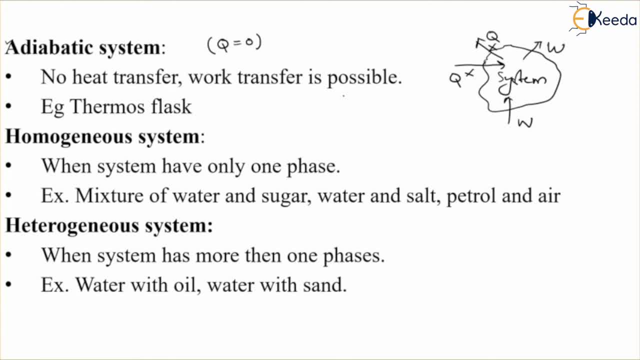 hot water or hot tea in thermos flask. So neither the heat is coming out from the thermos flask to the surrounding nor any kind of heat transfer is possible from surrounding to the thermos flask. So this is the example of adiabatic system. Now let's see another type of system, that is 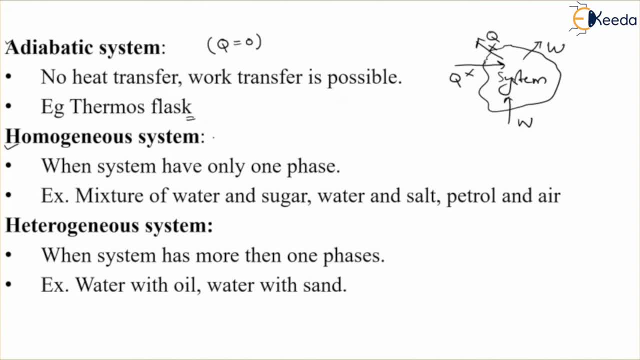 homogeneous system. So this homogeneous system is based on the chemical composition and physical structure of the system. So it is defined as a system when the system have only one phase. So this one phase is representing the physical structure, It is representing the physical. 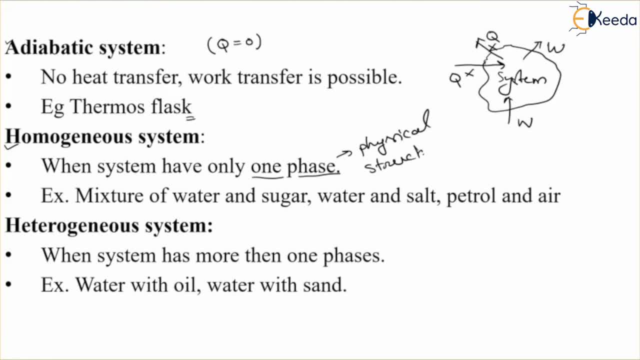 properties or physical structure of the system. and this physical structure we are not defining on the basis of one substance. We are defining this physical structure on the basis of mixture of the substances. So if the system have only one phase, it can be the mixture of number of. 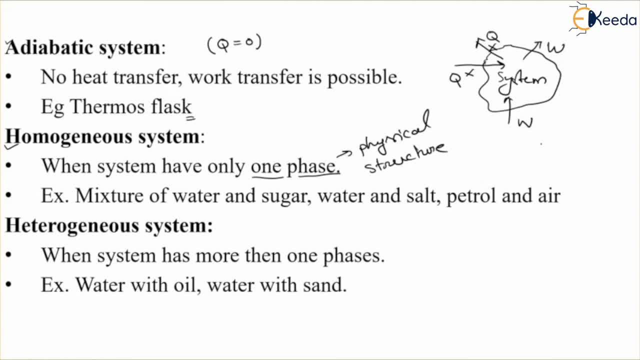 substances, but the phase will be uniform. Suppose if we have water and if we are adding salt into the water. so the color of the water will be same and the physical composition will not change. Here chemical composition can be same or it can be differ, but physically it will. 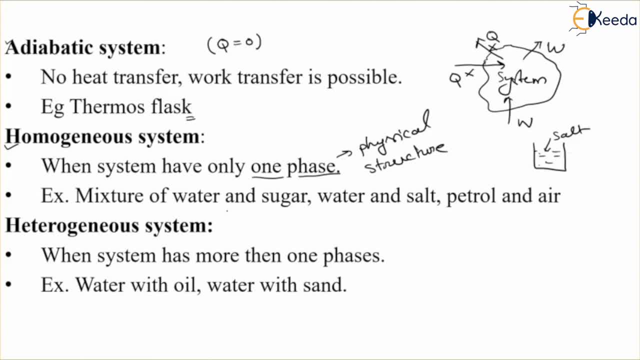 look same. So example of the homogeneous system we can take as mixture of water in salt, water in sugar and other example we can take in IC engine. petrol in air mixture is also considered as the homogeneous mixture. So these are the example of homogeneous system where chemical composition. 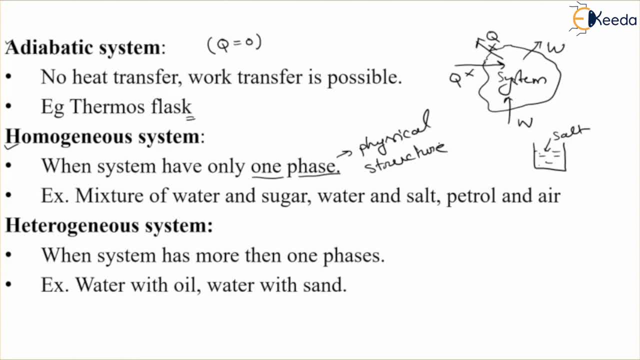 can be same or can be different, but the physical structure will be same or the system will have only one phase. So this is about the homogeneous system Now. next is heterogeneous system. So heterogeneous system is just opposite to homogeneous system when the system has more than one phases. If we are considering 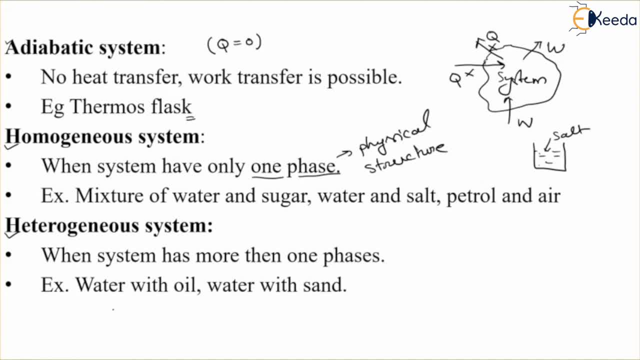 more than one phases. so as an example we can take the mixture of water and oil. If we mix water and oil together, So because of the density difference, we can easily discriminate between water and oil. Because of the density difference, oil will be on the upper surface of the water. or if we mix water.